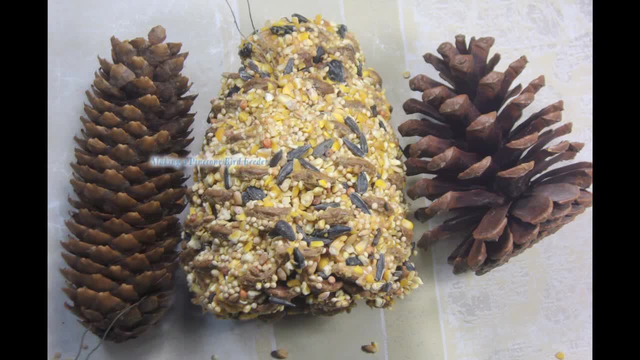 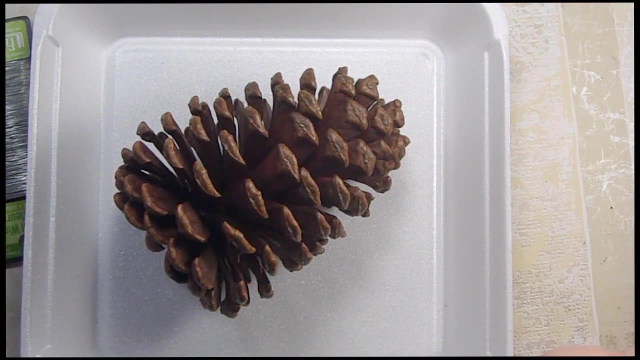 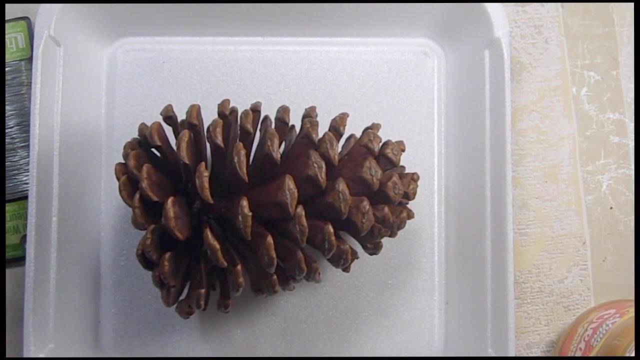 Hi, it's Sandy Parker, and welcome to Crafting for Almost Everyone. Today, we're going to make our birds a Christmas present. This is a huge pine cone. I'm going to measure it for you because it is huge. It is roughly a six inch long pine cone. 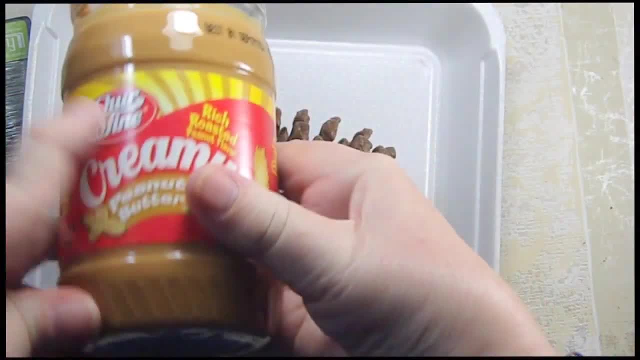 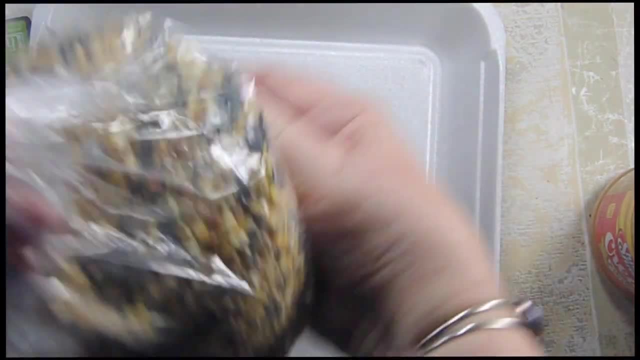 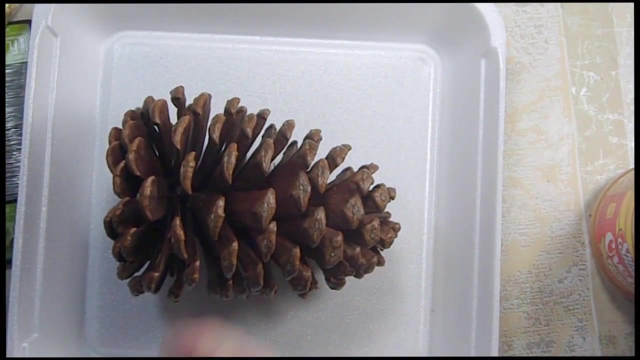 We are going to use cheap generic creamy peanut butter, Not chunky creamy peanut butter. And I went to the bulk section of my grocery store and I bought bulk bird seed. that was like 48 cents a pound, So this was 48 cents worth, or roughly 48 cents worth. 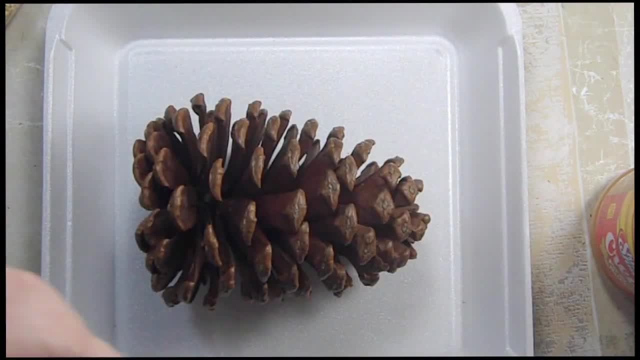 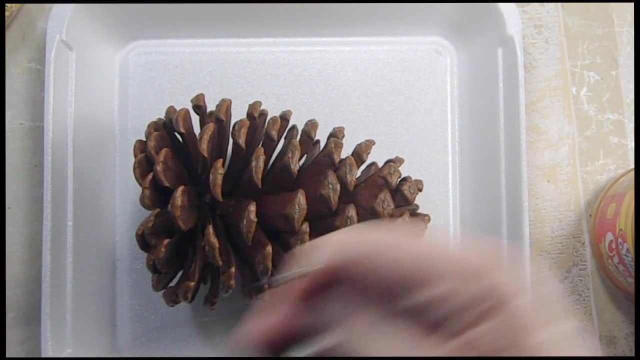 And I'm going to use some floral wire. This is I don't know. it just says floral wire. It doesn't say anything like how many gauge or whatever, And I think I'm going to wire mine up first. What I'm going to do is I think I'm going to wire into the top here. 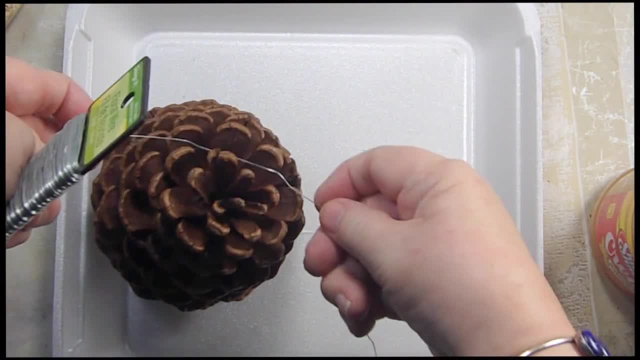 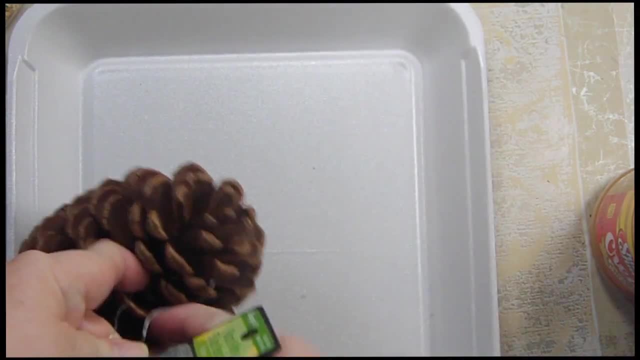 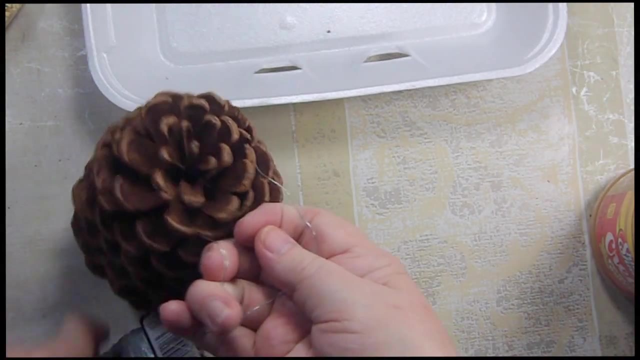 Just so I'm sure that my pine cone is going to hold up. you know, with the birds, My bird feeders, two of my big ones got ruined By the neighborhood bear. I live very, very close to a town, but apparently this bear doesn't care where I live. 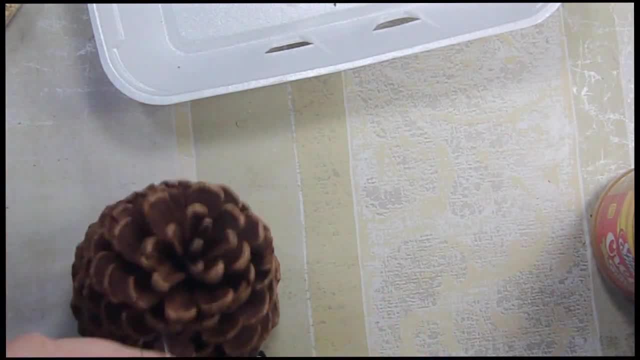 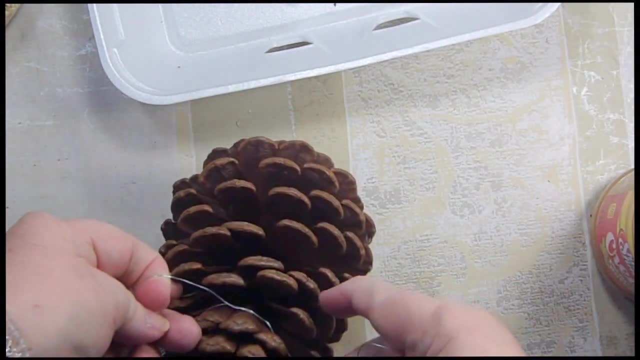 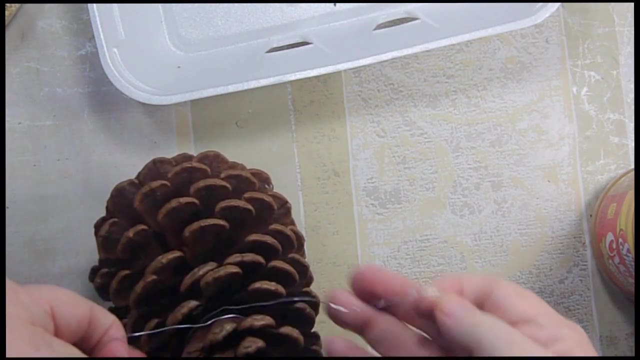 It's all about what's for supper Sandy, And so, anyway, it ruined three of my big bird feeders, And so now I'm going to go to the natural one so that hopefully, he doesn't destroy a bunch more. Okay, so before I go any further, I'll just show you what I'm doing. 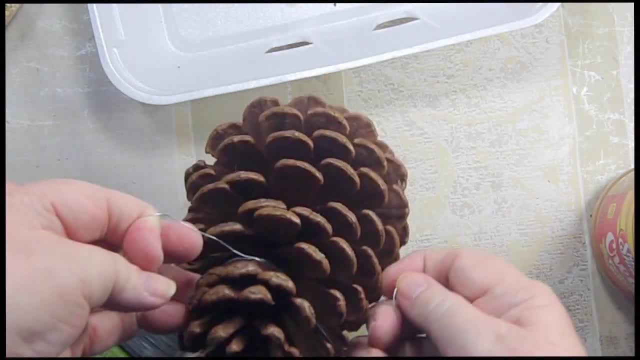 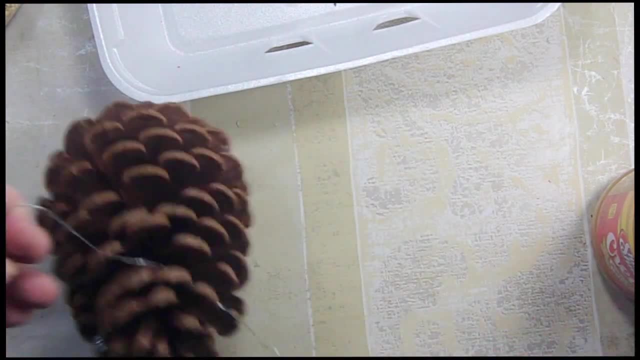 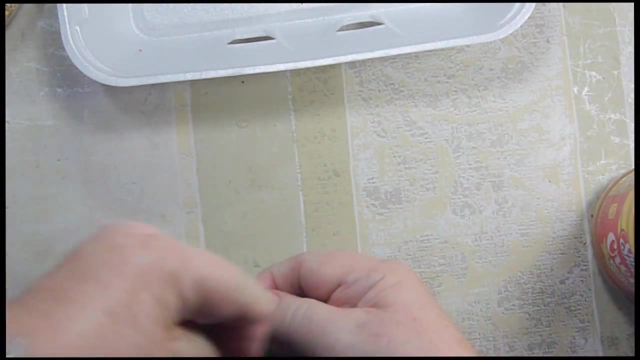 I wrapped the wire around about Three or four rows down And I'm just going to. I have it, I just have it. let's see. I have about a foot on this end And the other end I have attached still to the wire, you know to the ream or whatever you call it. 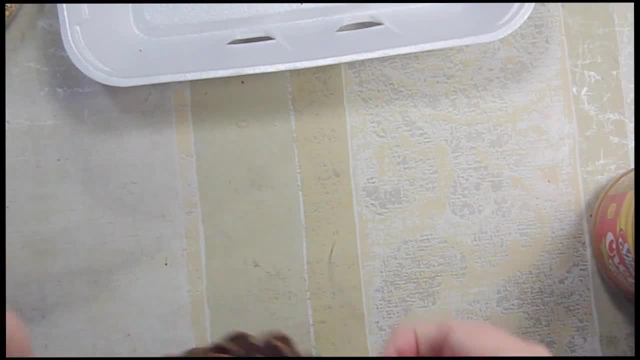 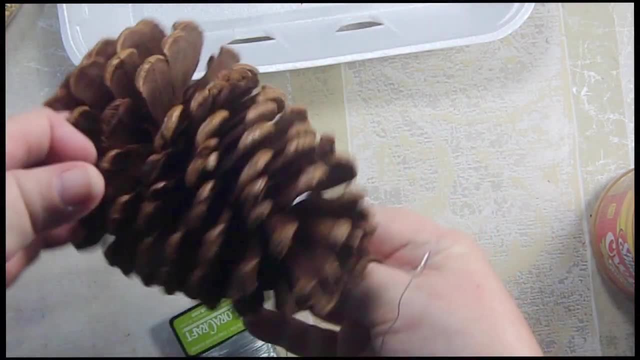 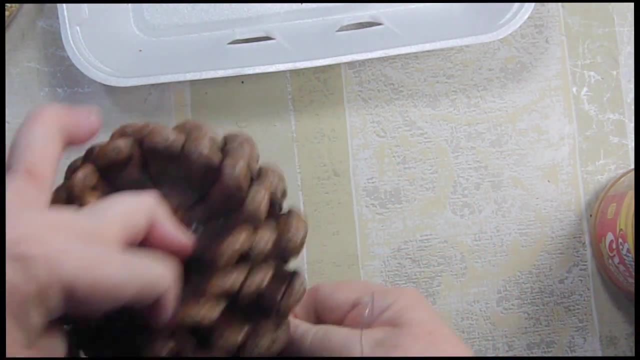 To the. you know whatever, We'll just call it the whatever. So I have that. I'm going to just twist it Once. I have it spun once, I'm just going to keep twisting it. I'm just going to keep twisting it to the side there to make sure that my wire is nice and tight like that. 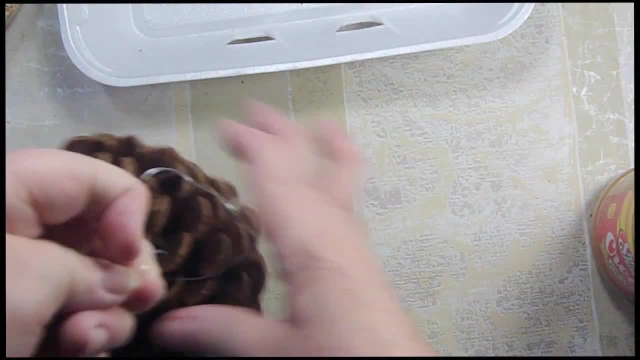 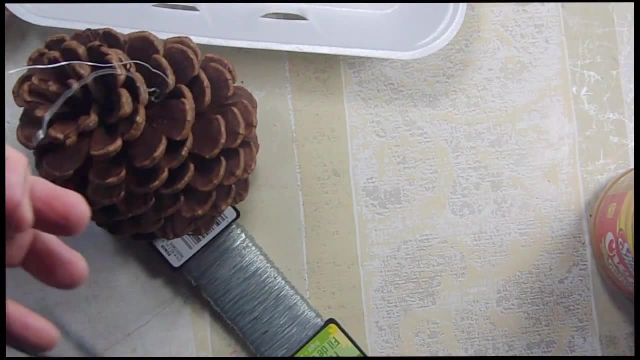 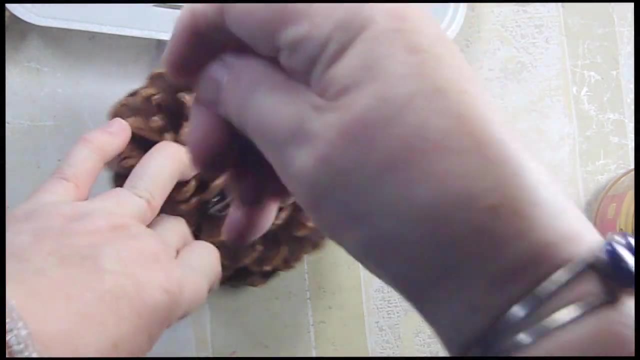 Then I'm going to take both ends of it like this And I'm going to cut off. let me get my scissors. sorry, One thing I forgot: my Tim Holtz scissors don't cut through anything, And so I have about a foot- whoo sorry about a foot- extra on both sides. 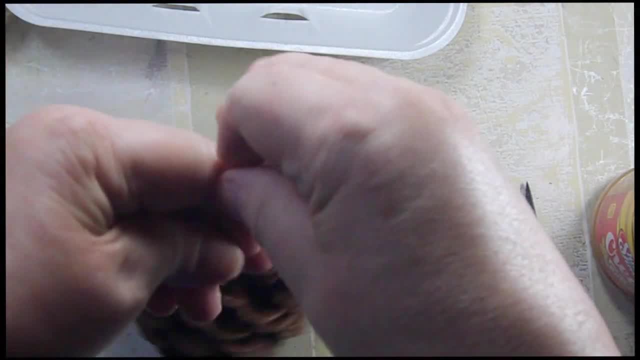 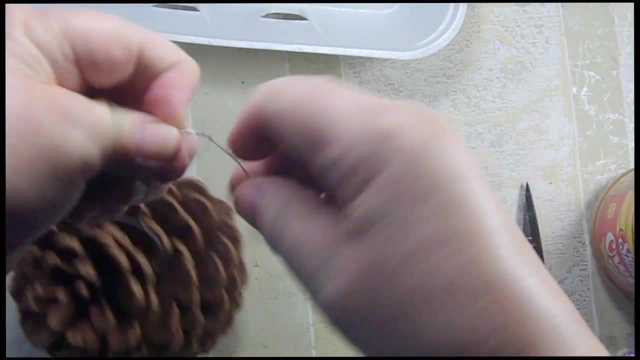 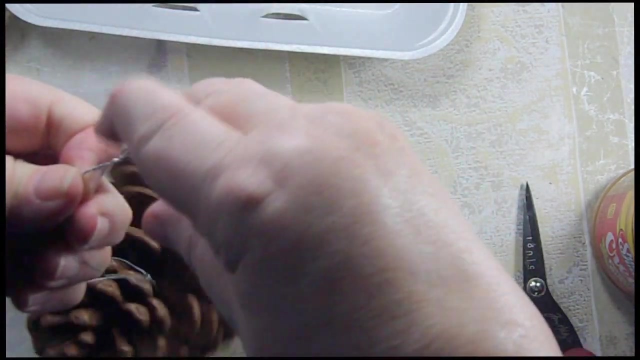 And I'm going to, I'm going to tie those into a knot. well, not tie it, I'm going to twist it into a twisty knot Many, many, many times. And then, when I'm done- doing that because it's you know, I don't want the ends- to cut my birds. 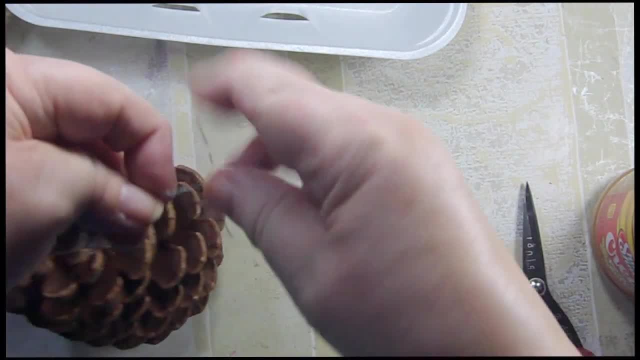 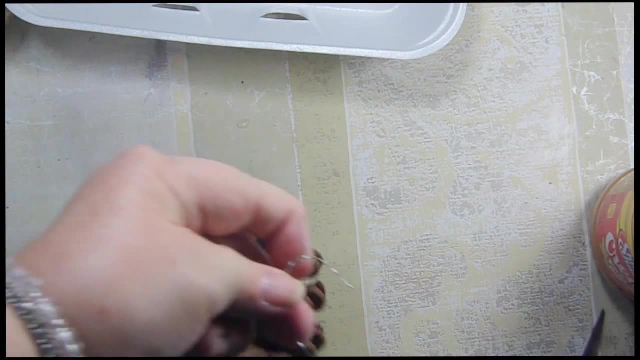 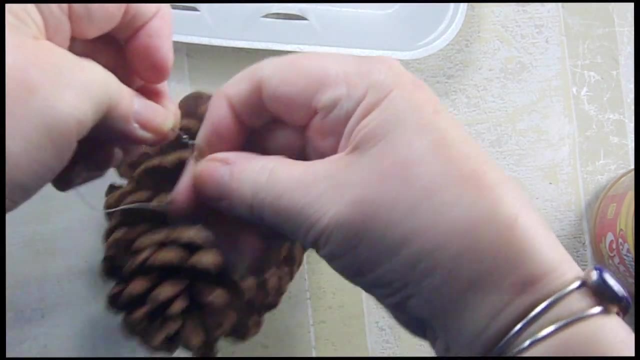 What I'm going to do is, once I get down closer to the end- and I'm sure that it's really well adhered like that- I'm going to snip off the edges that are sticking And then I'm going to turn that piece in and I'm going to twist it back on the circle. 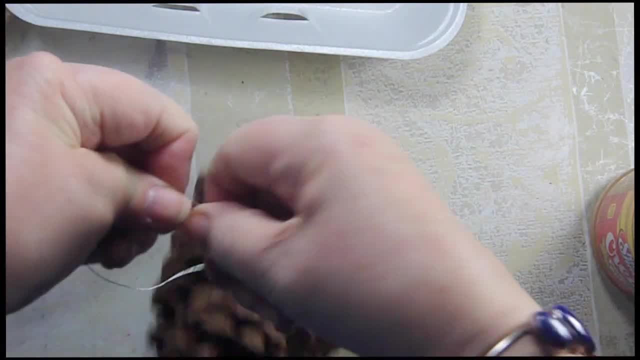 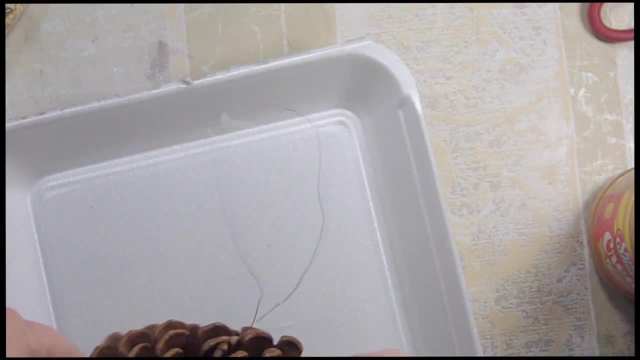 Can you see what I'm doing? I'm twisting it into the circle that I just made. So now that we've got it completely wired up and ready to go, the wire should stay, because the birds aren't going to, you know, be overly heavy on it. 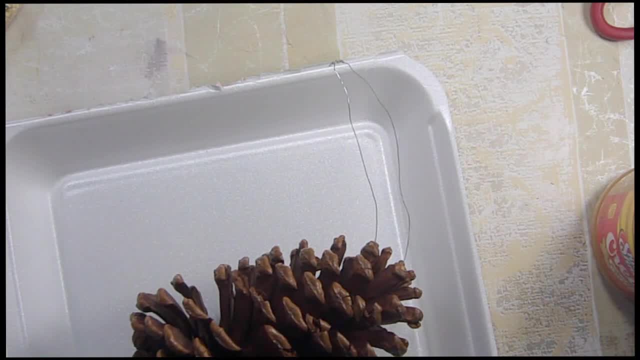 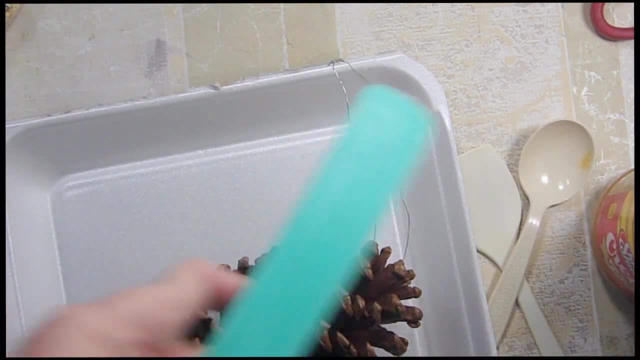 I'm going to use a couple different tools to spread my peanut butter. Okay, I have this spoon and I have this spatula and then I have a smaller one, So I thought I'd start with the spatula. that's rubber or rubbery. 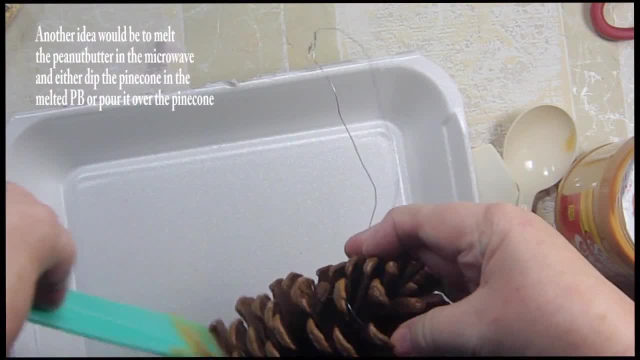 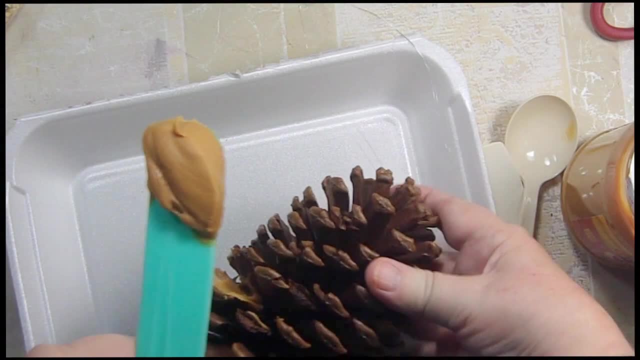 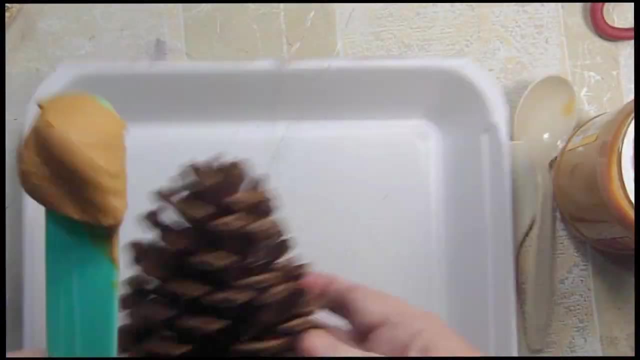 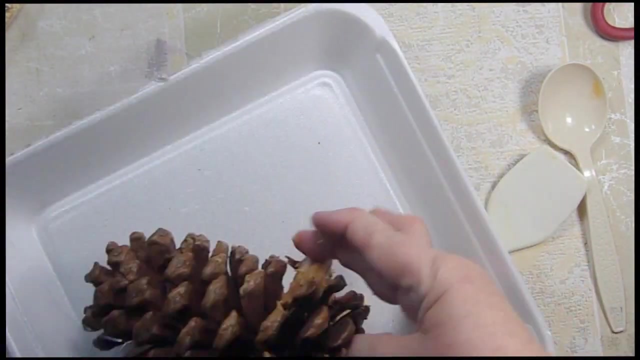 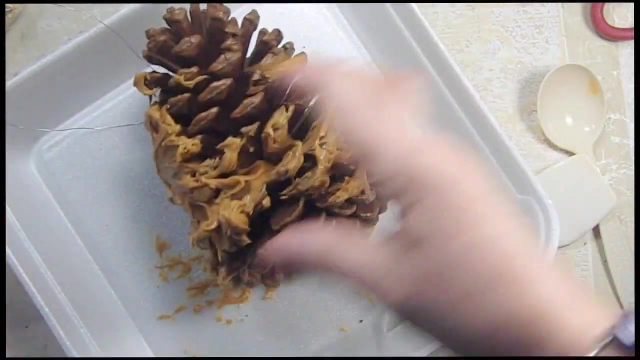 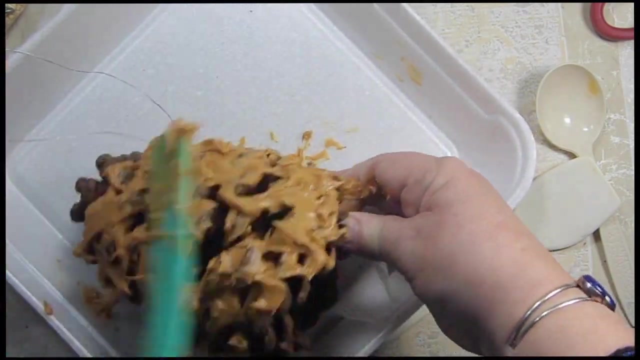 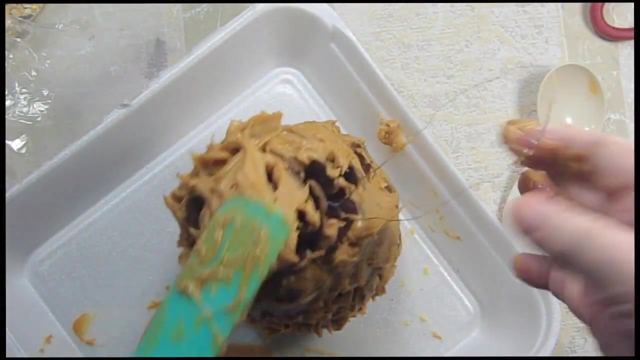 and see if I can kind of get back into the grooves with it And I'm going to use the spatula like I'm kind of buttering, no more like I'm baking, doing something with a cake. See the reason I did the wire first. 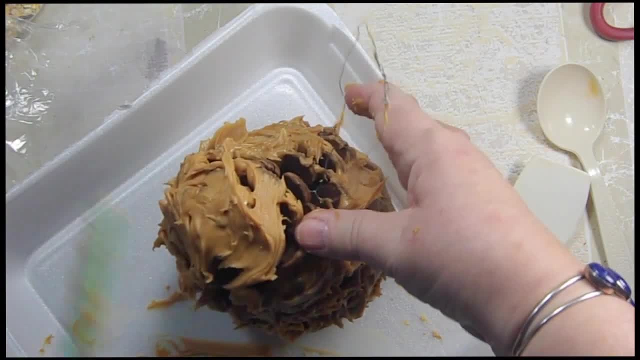 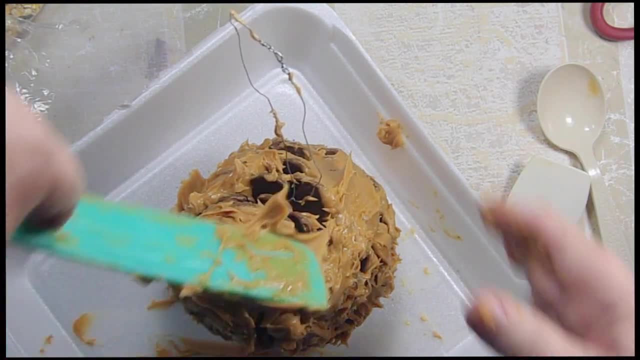 If I hadn't done the wire first, I would end up with trying to work around the peanut butter and I haven't gotten to the birdseed level. but if I had had my birdseed in here, putting the wire in after the fact would have been gross and not too much fun. 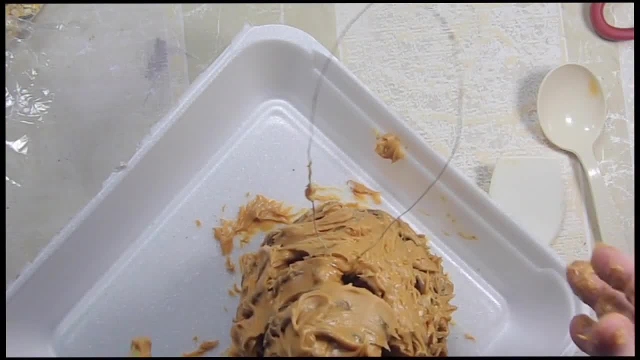 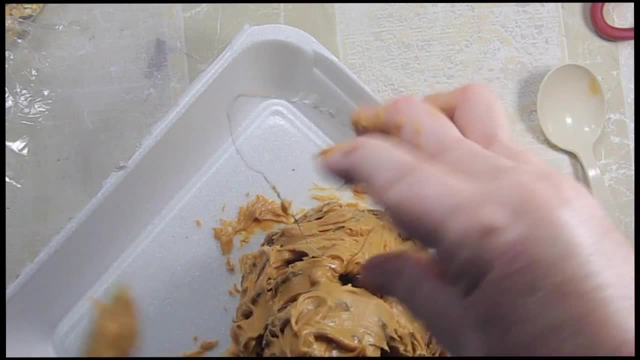 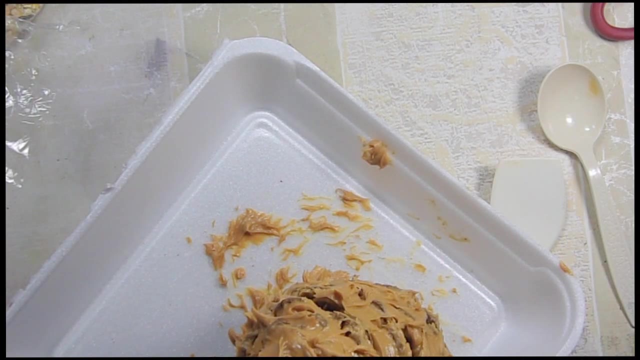 I have a very, very serious audience right here now. My dogs are just very, very quietly sitting behind me waiting for me to go. Okay, let's have some peanut butter. I think we're pretty good. I would clean my hands now, but what's the point? because we're going to have birdseed all over them now and peanut butter. 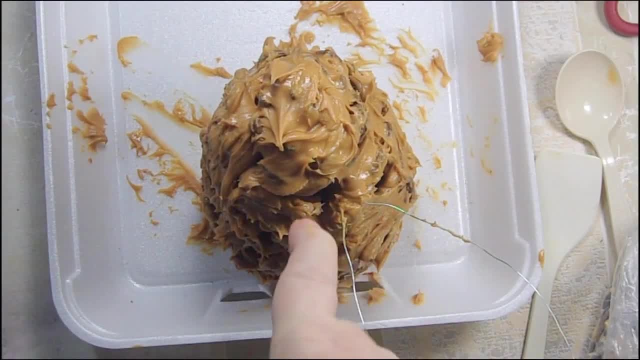 So hold on for just a second and let me get my birdseed open. Well, if it wasn't in the screen for part of that, I'm going to have Rich cut out any part where the pine cone getting slathered with peanut butter wasn't in frame. 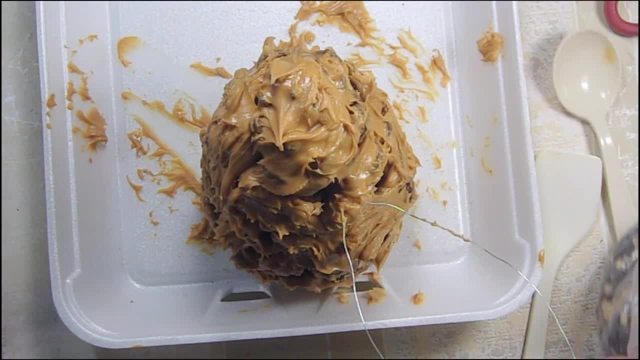 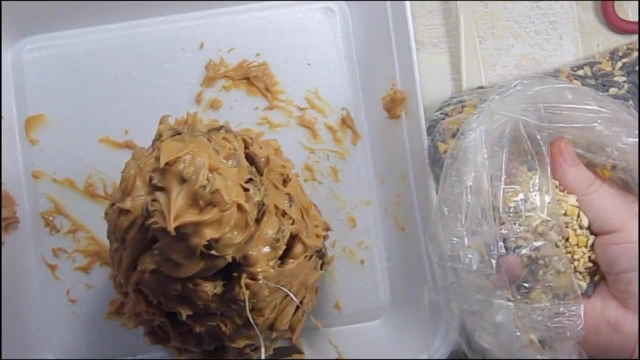 because I mean, if you saw any of it, you saw enough to know how to do it. I have my bag of. Let me see if I can have it. Yeah, I have it in there. I want to see if you can make sure you can see that. 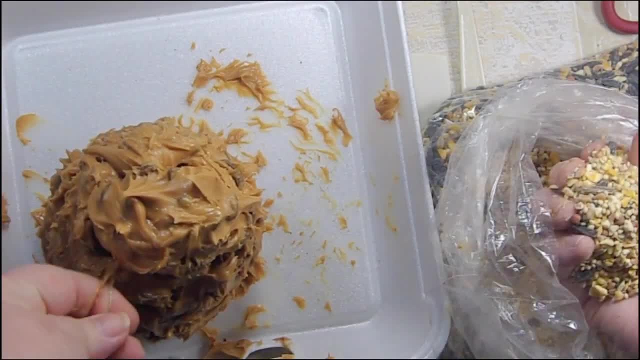 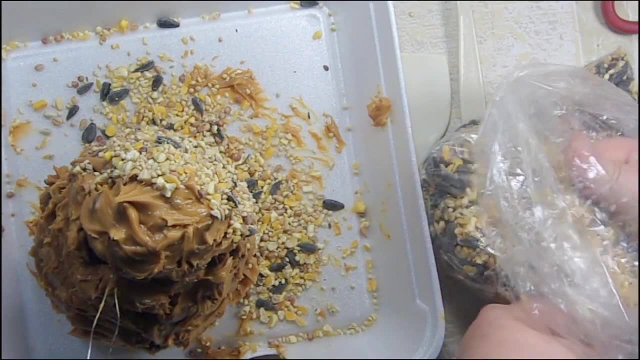 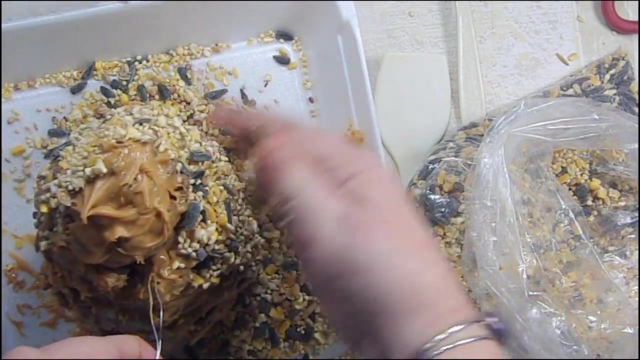 I'm going to hold on to my pine cone by the wire, just so I have a little bit of stability, and then I'm just going to pat birdseed into the side of it. I'm going to turn it. Well, now I've got some action. I've got Honey. 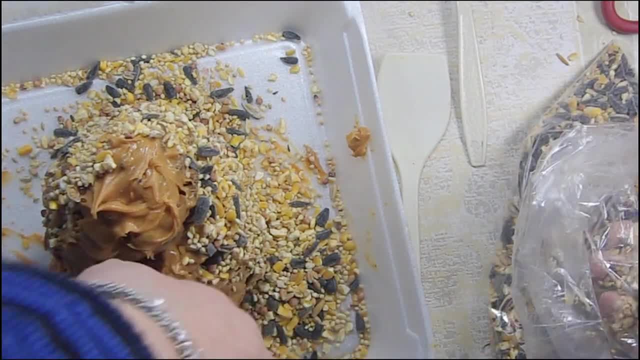 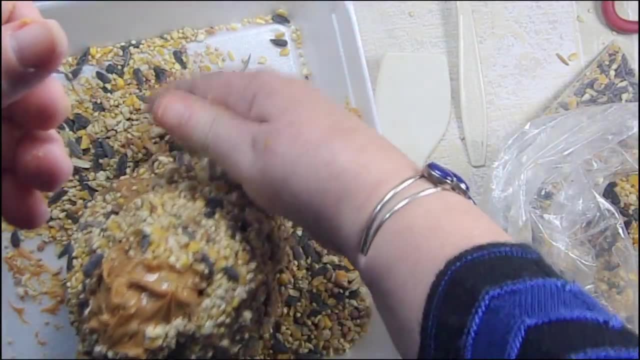 Honey's now decided there's got to be a better way to get to that peanut butter. She's right beside the peanut butter now. In a second she'll probably be in the frame. This takeout container has worked pretty well so far. 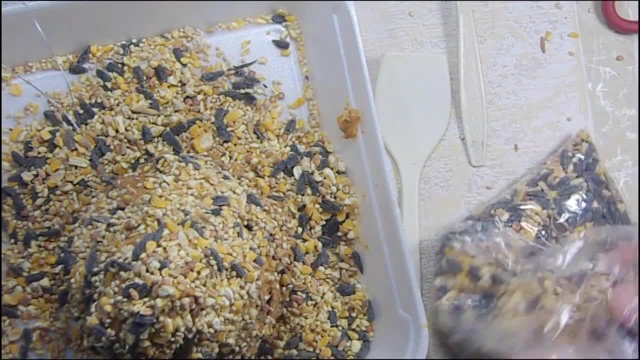 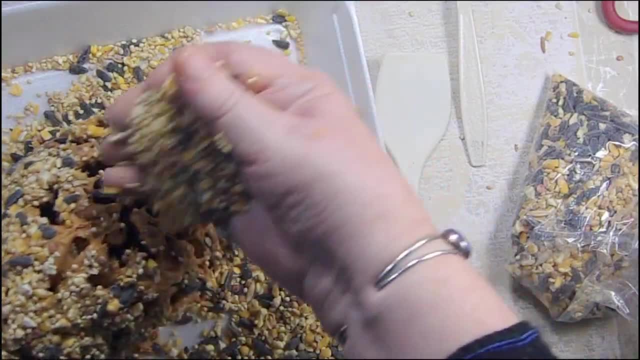 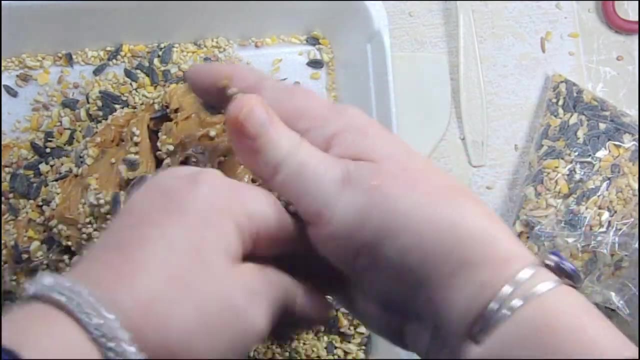 I'm hoping that it'll continue to work, that it won't snap. I don't think it will. I'm going to turn it so I can get into this side area. Okay, I'm going to lay it on its side And. 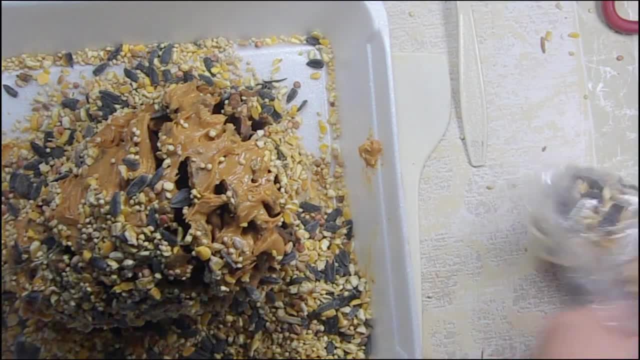 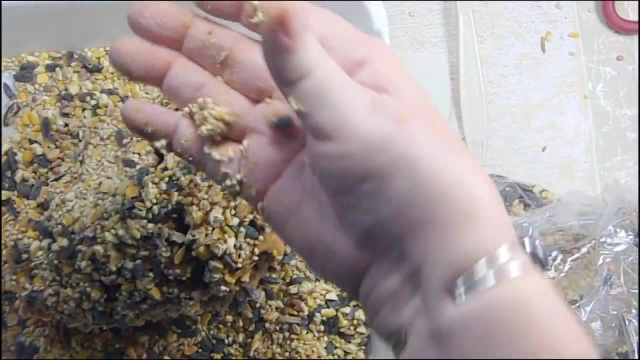 I think I'm going to dump some of the you know, put more on it and then, after I put more of this on it, then I think I'm going to roll it in the peanut butter or in the birdseed that's left behind. 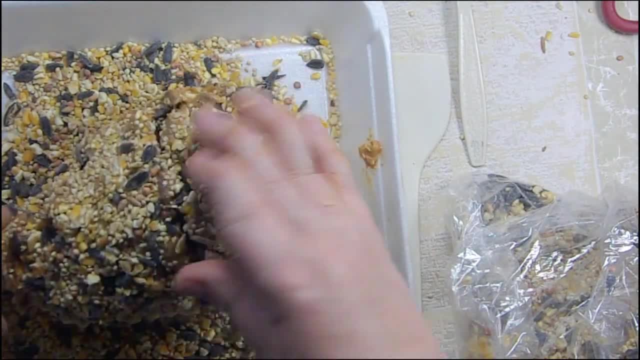 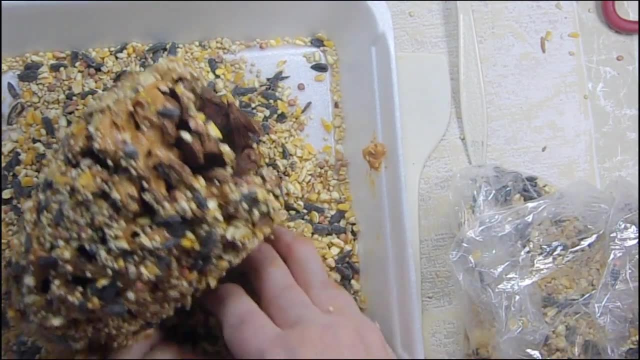 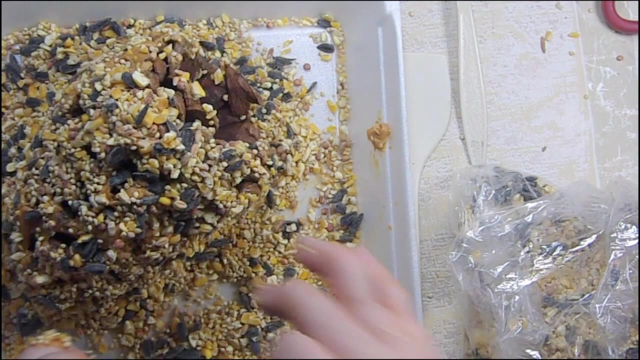 So I'm tapping it nice and gently. The goal obviously is to make sure that I cover the whole um, everything that's sticky, and that I don't end up with anything that's not sticky. You know I don't want to. I mean, I don't want to have any of the 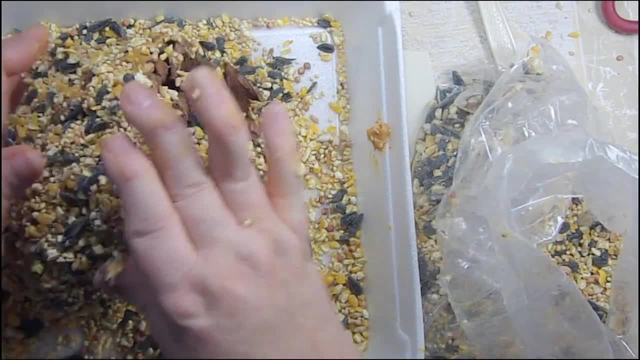 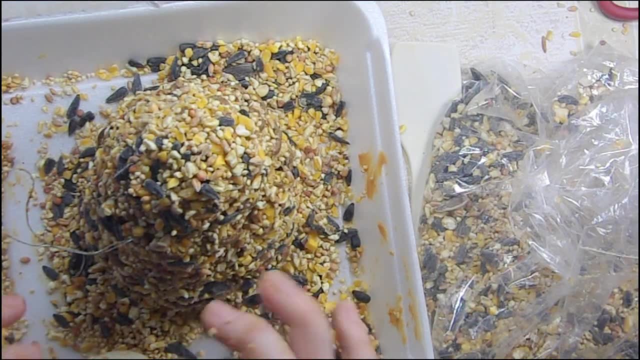 any of the sticky peanut buttery part that's not covered I want to cover. So let me get my my uh mess off and we'll see how how our little project came out. So that's what it looks like after it's done. 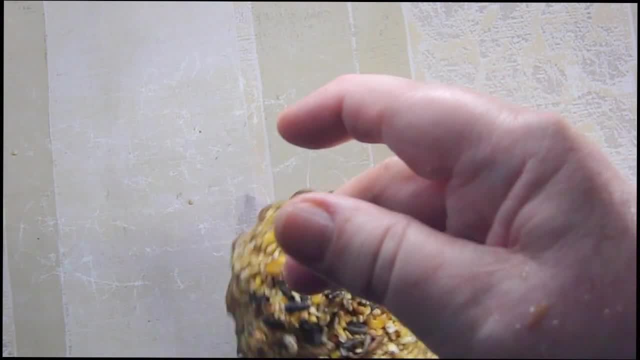 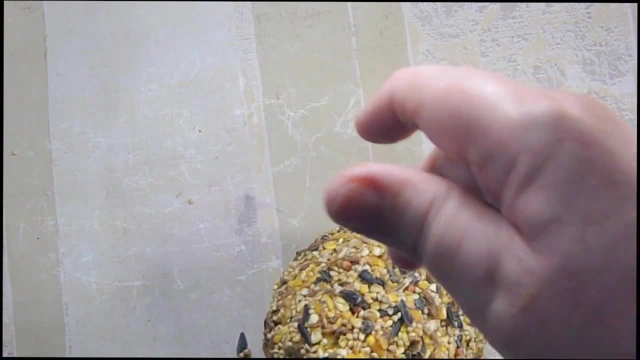 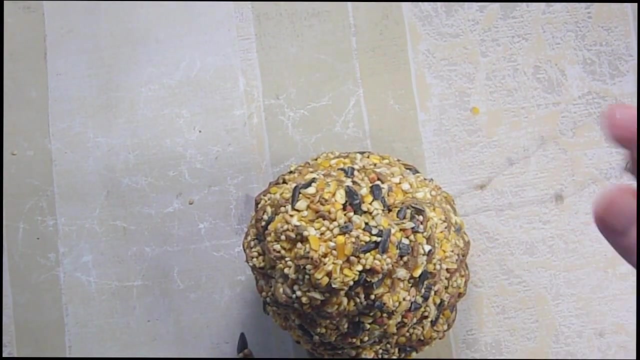 And I put it in the refrigerator so that it is the, the peanut butter and the- uh, you know it, it held better. And then I'm just going to hang it outside. I'm going to hang it outside on um, I have hooks to hang, you know, like those um shepherd hooks. 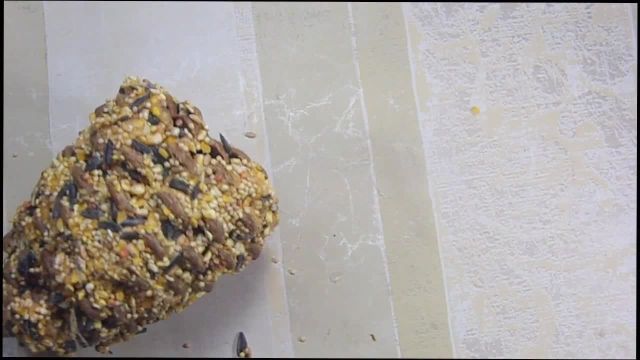 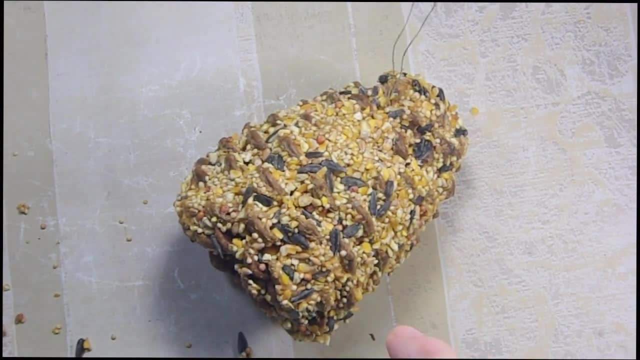 I have one of those. I'm going to hang my big pine cone on There. it is sideways And I think it came out really well. And these are not inexpensive to make because, well, when you use a pine cone as big as mine, 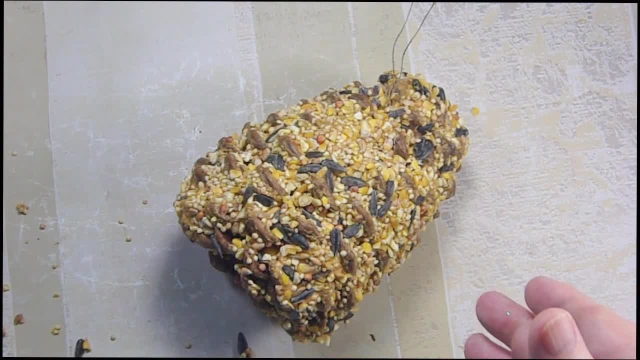 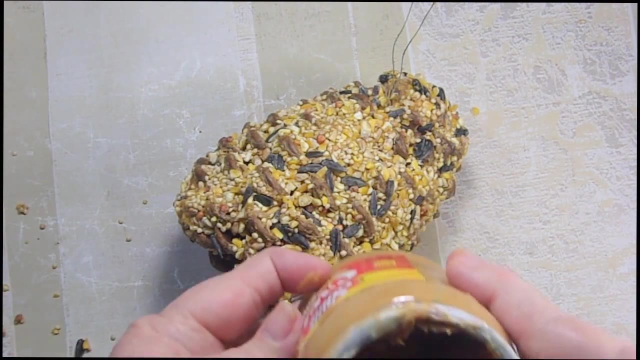 um, it took almost a whole jar of $1.50 worth of peanut butter and, uh, about, I don't know, let's say, a half of a pound of the bird seed. So there's about, oh no, there's, um, there's maybe a third, a quarter, maybe a quarter of a jar of peanut butter. 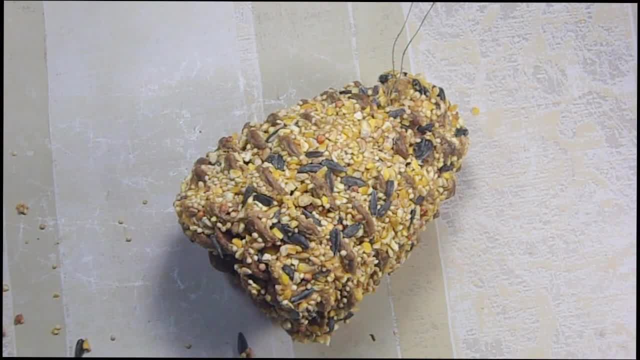 So there's at least- uh, there's at least- a dollar and a quarter involved in making one when you're using a pine cone as big as mine. But I do think it would be a fun gift to give to, like a grandmother, for kids to make. 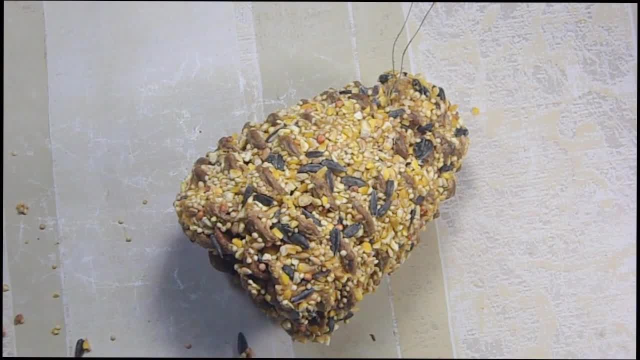 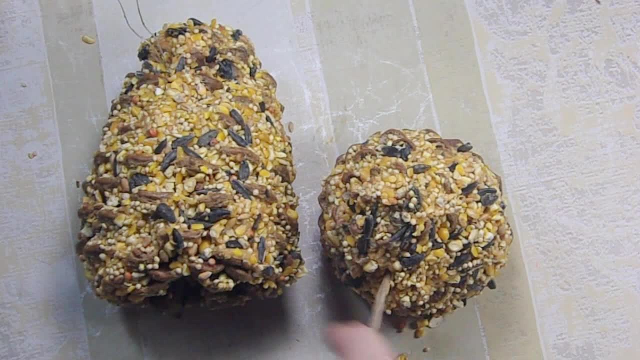 It's easy to make and it'd be fun for you and your kids to make over Thanksgiving break. So I made my second one, And on this one I used, like a jute, thicker twine and I just tied a knot in it. 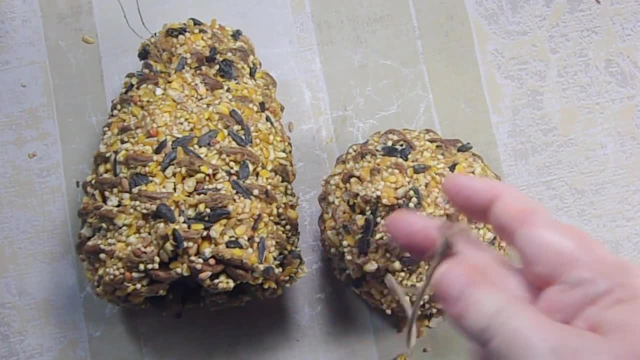 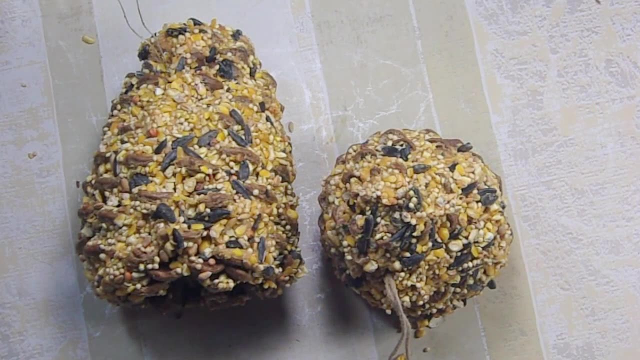 And I like this better. Again, it's not going to hold up long term, but for one round of birds eating the seed and the peanut butter, I'm sure it'll hold up that long And, um, we're supposed to get like 15 to 18 inches of snow in the next three days. 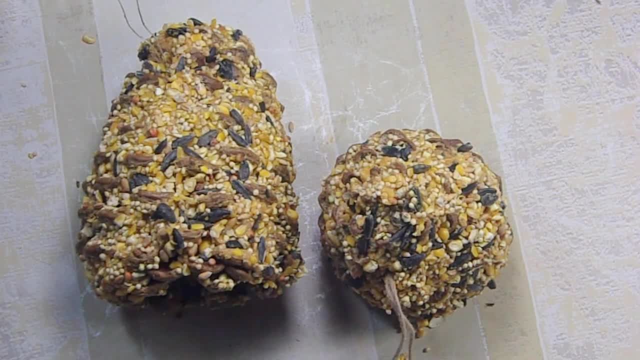 So it's more important than ever that I feed my bird. I hope you enjoyed this video and that you give it a thumbs up and subscribe And tell your friends about me on social media, because I really appreciate that. And thanks so much for watching. Bye-bye.